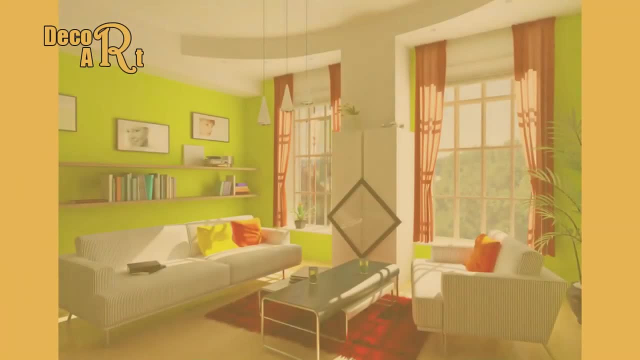 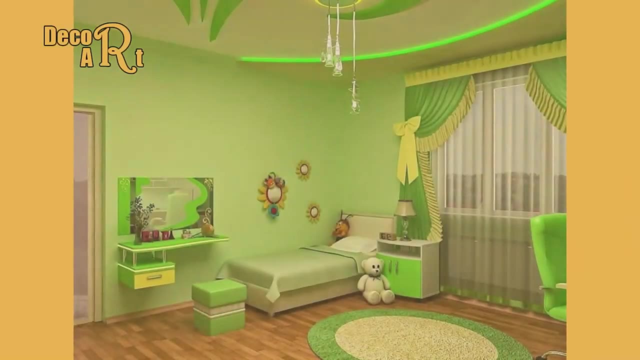 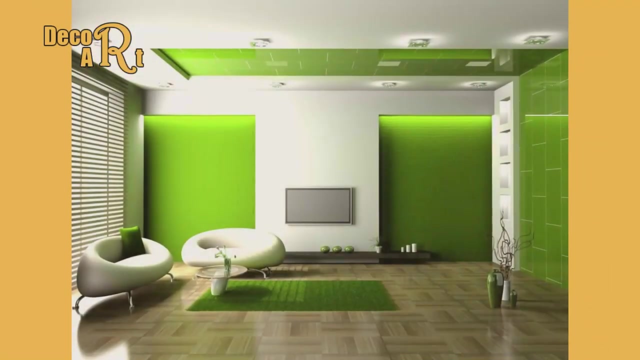 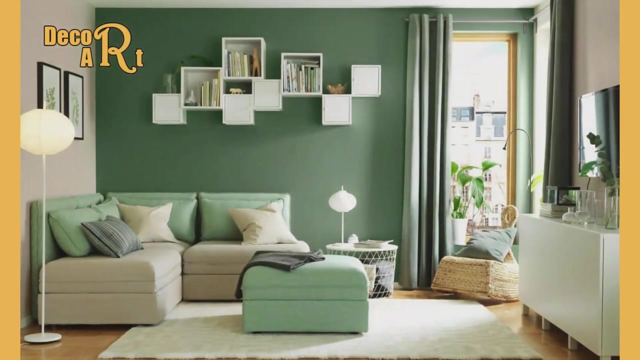 Green in interior design. If you want to make a large space more pleasant, you will achieve this using green carpets or painting green walls. Green furniture always looks good. If you are not sure where and how to use green, try with green details. A few well-placed vases or green pillows will freshen up your home. 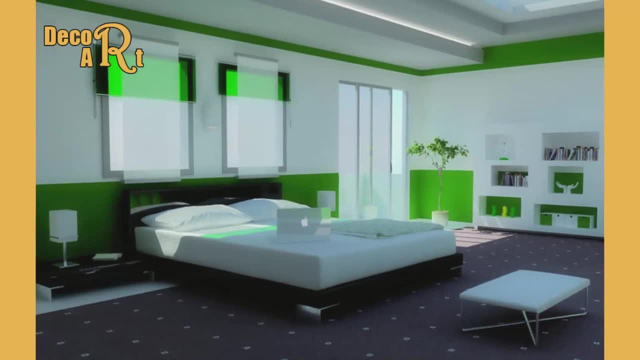 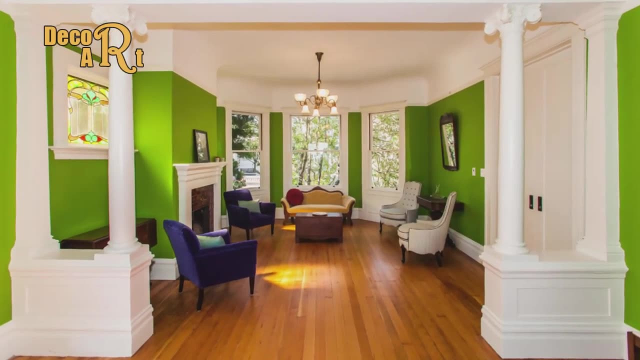 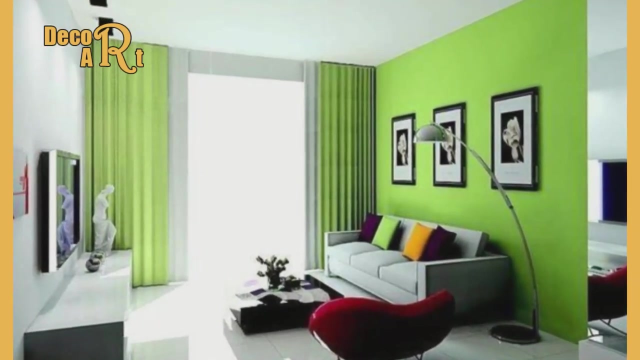 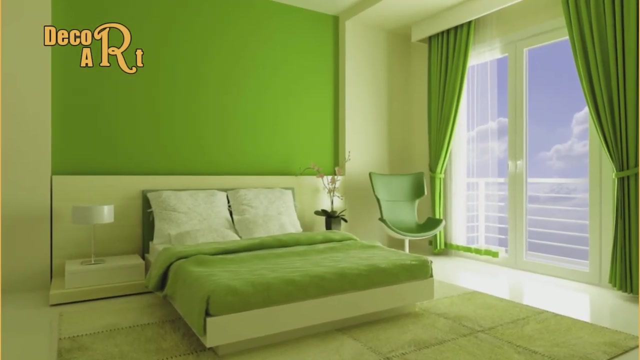 When in doubt, plants and green furniture can be used. Green flowers decoration is a fantastic idea, but do not overdo it. The most important characteristic of green color is its multi-purpose hues. If you are wondering whether it will fit your space, the answer is usually yes. 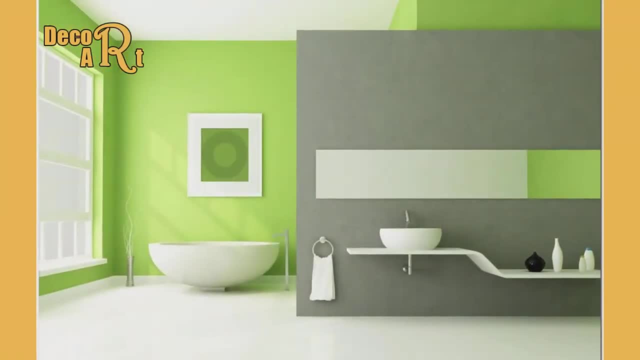 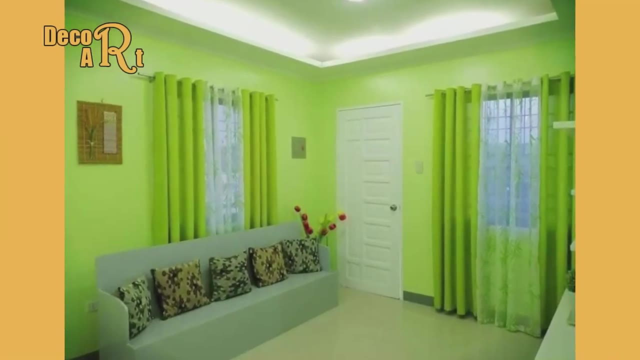 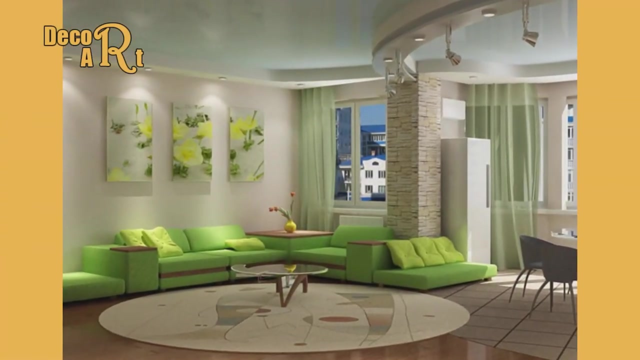 Whether it's a green accent wall or a few seafoam green throw pillows, adding a pop of green will make your home look more beautiful. Green has the power to completely transform any room. If you want a more dramatic feel, be sure to indulge in colors like dark moss and emerald. 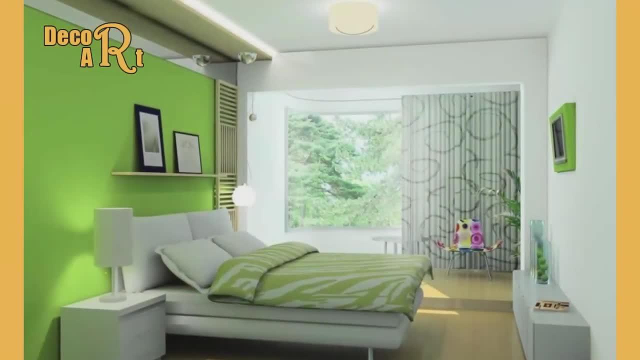 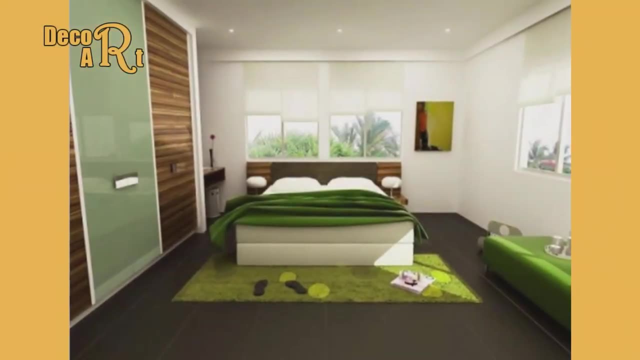 Green is the color of your home. Looking for a little tranquility, Paint your walls in a soft tissue like mint. And for those looking to make a big impact, there is always the tried-and-true lime green. Green is the color of your home. 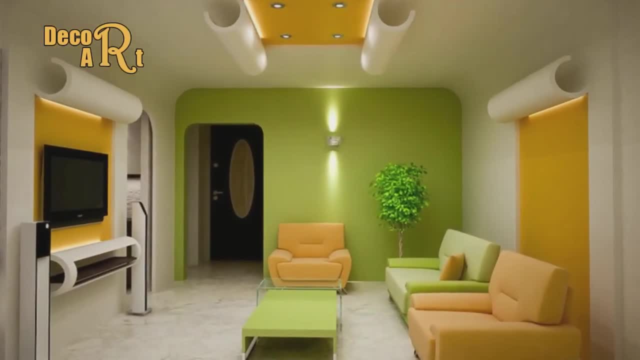 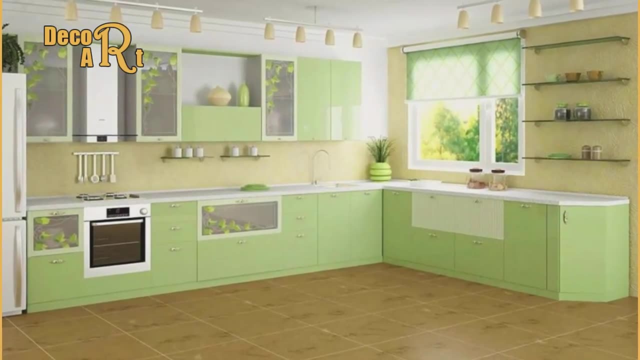 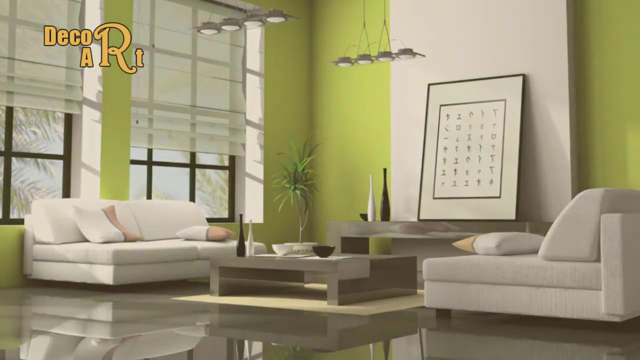 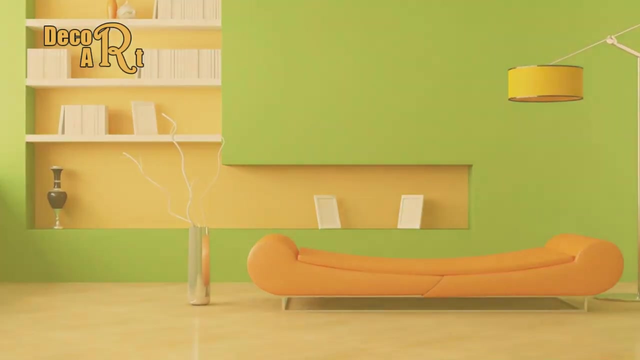 Green is the color of your home. quite sure which color best suits you? we've got you covered. Keep scrolling to see our hand-picked collection of the best green living rooms by designers and visualizers around the globe. There are several colors that look fresh, but green is in the first place. 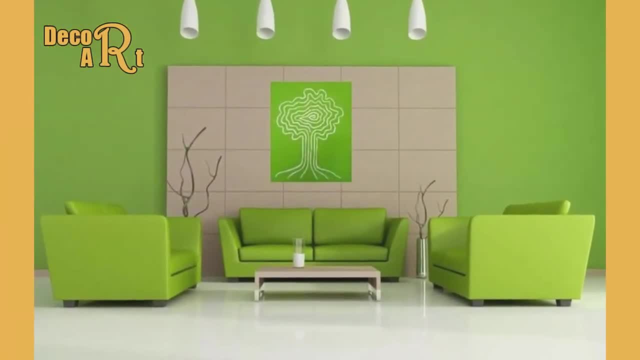 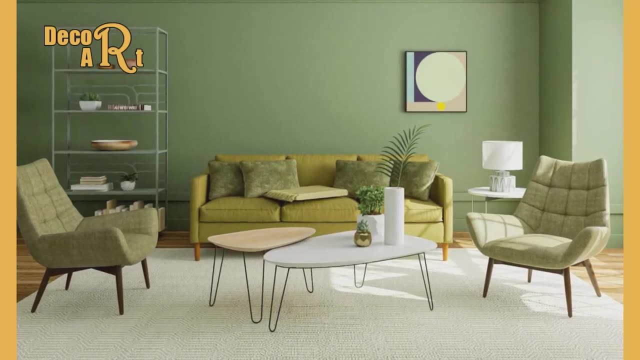 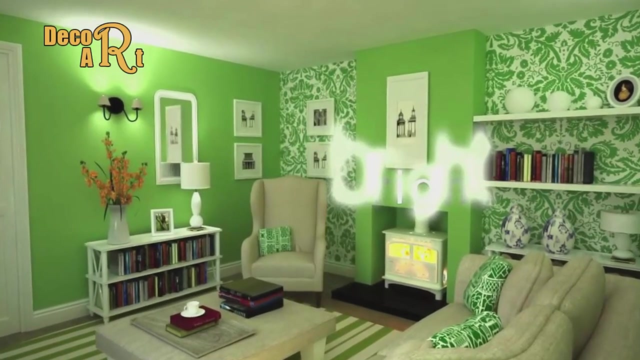 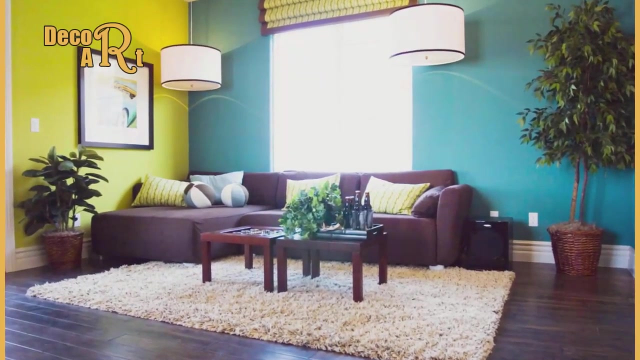 Green is the color of renewal and growth. it has soothing characteristics. Due to its characteristics, designers often use it in interior design. It comes in a variety of shades from light green to dark green emerald. Since green is neutral, it agrees with almost all colors. 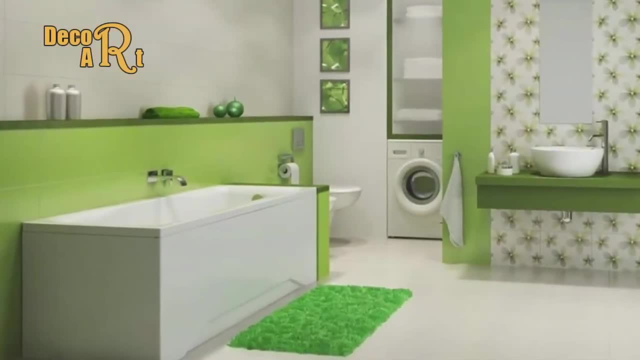 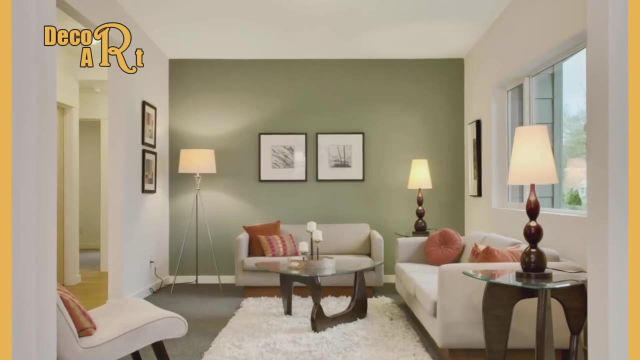 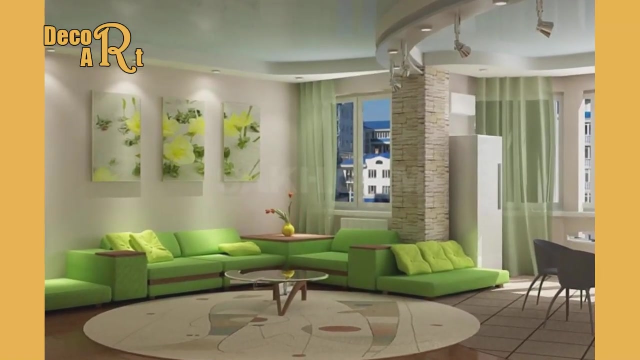 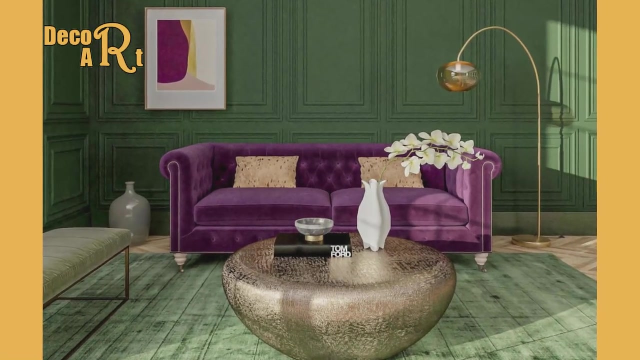 That is one reason plus why it is easy to use Green in interior design. If you want to make a large space more pleasant, you will achieve this using green carpets or painting green walls. Green furniture always looks good. If you are not sure where and how to use green, try with green details. 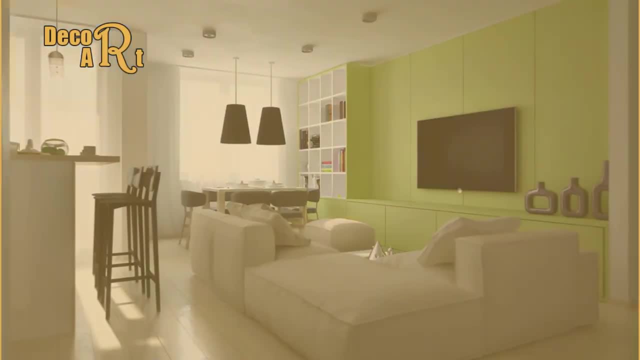 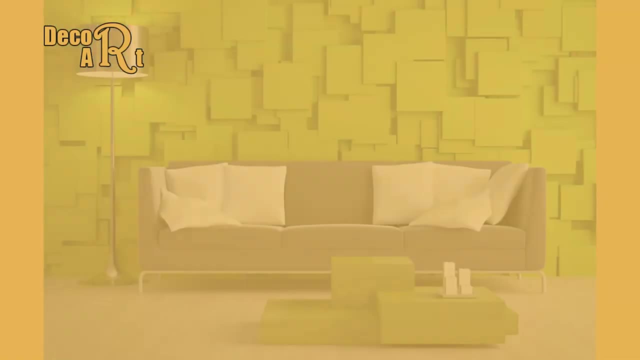 A few well-placed vases or green pillows will freshen up your home. If you are not sure where and how to use green, try with green details home when in doubt. plants and green flowers decoration is a fantastic idea, but do not overdo it. the most important characteristic of green color is its 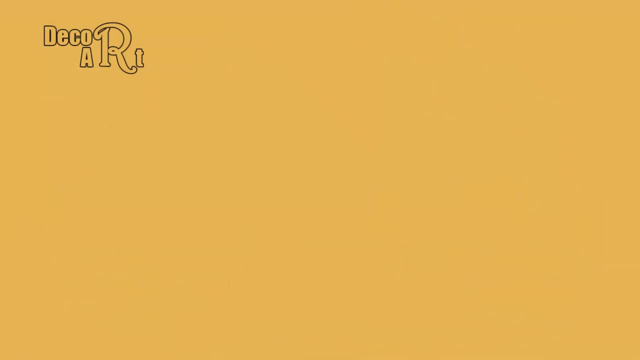 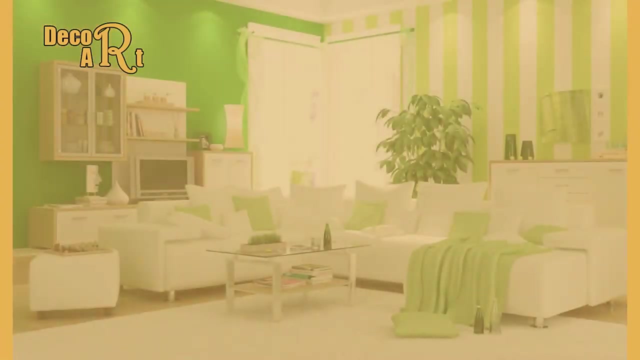 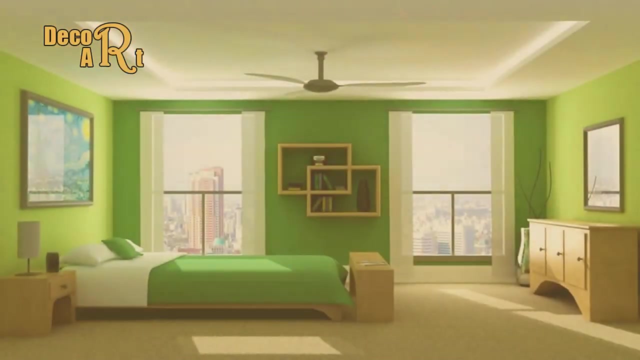 multi-purpose use. if you are wondering whether it will fit your space, the answer is usually yes, whether it's a green accent wall or a few seafoam green throw pillows. adding a pop of green has a power to completely transform any room. if you want a more dramatic feel, be sure to indulge in colors like dark, moss and 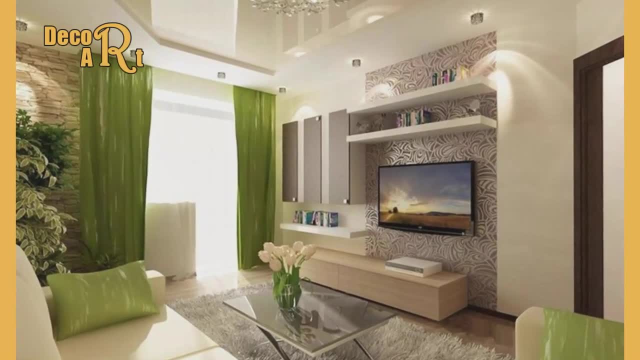 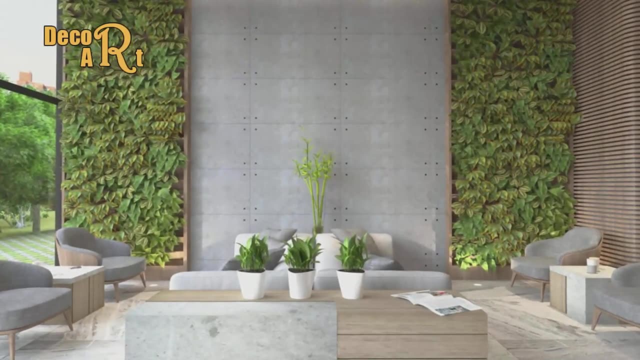 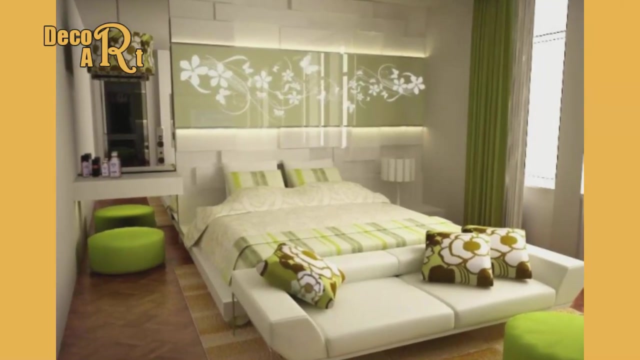 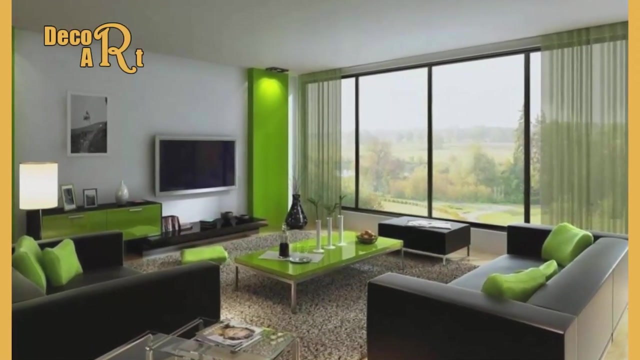 emerald green. looking for a little tranquility, paint your walls in a soft tissue like mint. and for those looking to make a big impact, there is always the tried-and-true lime green. if you're not quite sure which color best suits you, we've got you covered. keep scrolling to see our hand-picked. 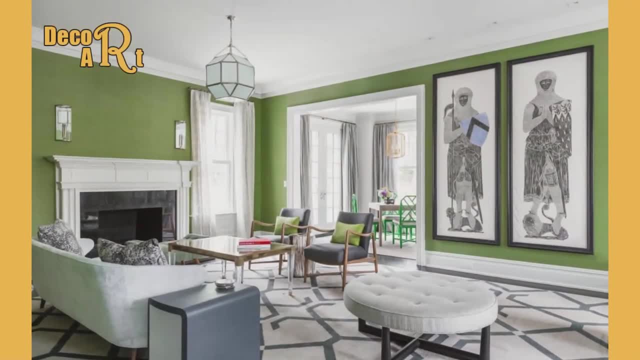 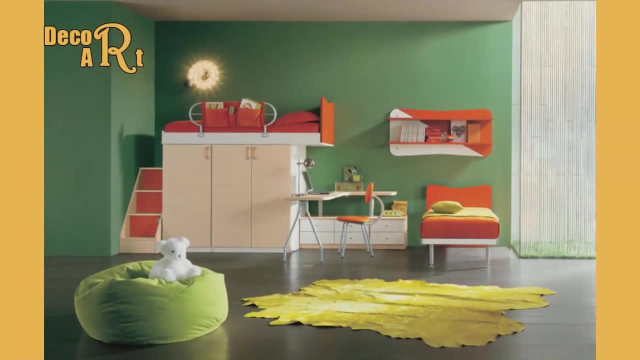 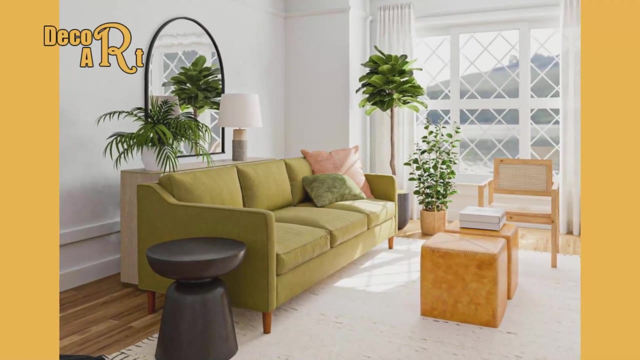 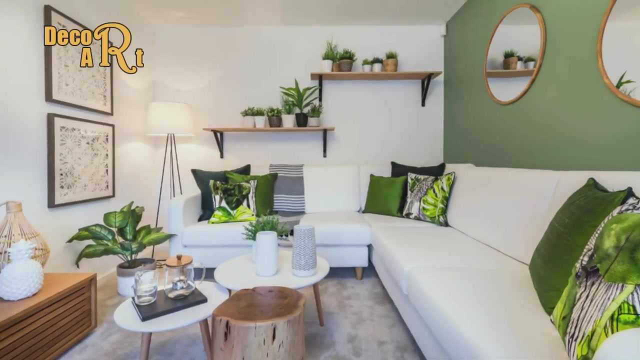 collection of the best green living rooms by designers and visualizers around the globe. there are several colors that look fresh, but green is in the first place. green is the color of renewal and growth. it has soothing characteristics. due to its characteristics, designers often use it in interior design. it comes in a variety. 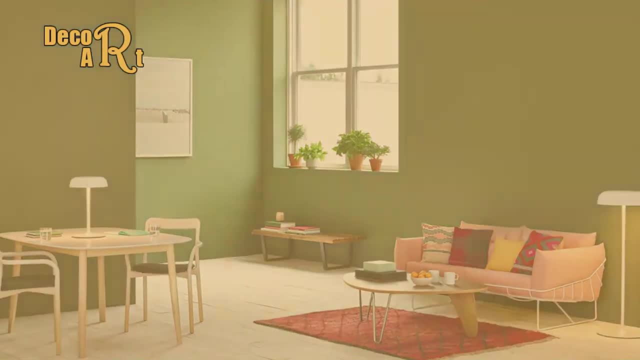 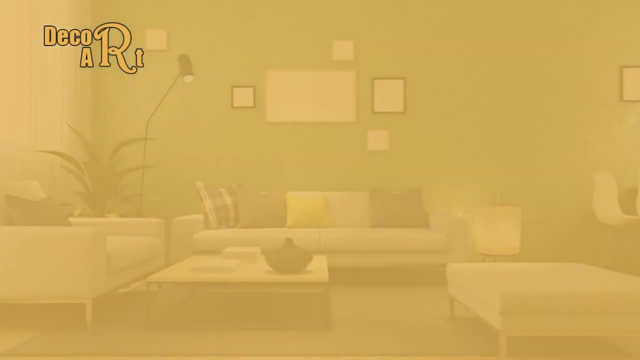 of shades from light green to dark green emerald. since green is neutral, it agrees with almost all of the other colors that are available in the market. green is a wonderful design for rough miniature or mold design. that is one reason plus why it is easy to use green in interior design, if you. 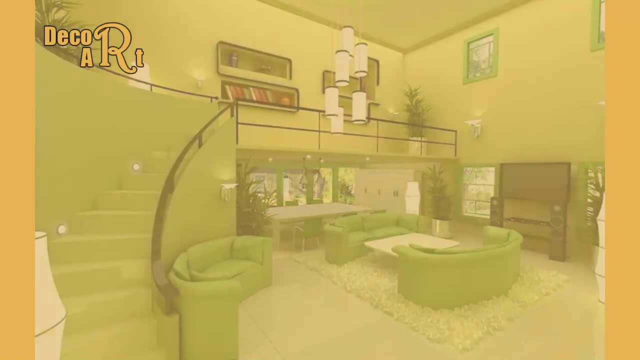 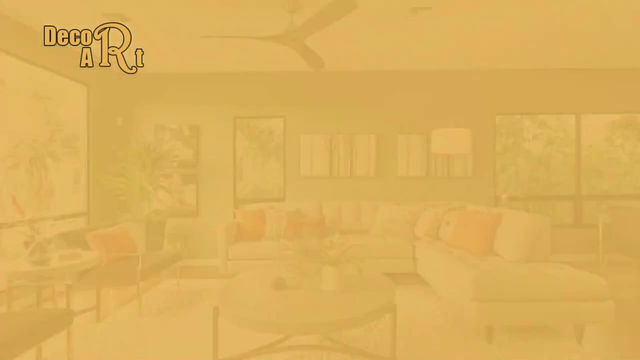 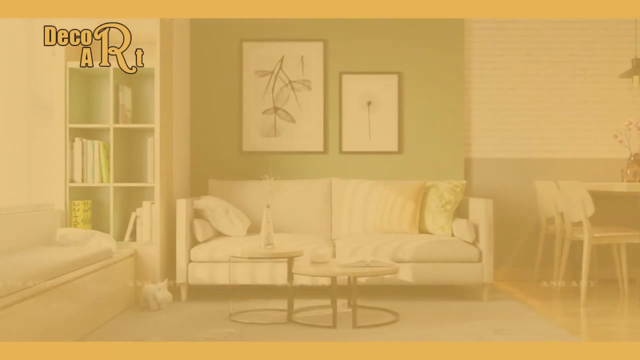 want to make a large space more pleasant. you will achieve this using green carpets are painting green walls. green furniture always looks good. if you are not sure where and how to use green, try with green details. few will placed vases or green pillows will freshen up your home when in doubt. 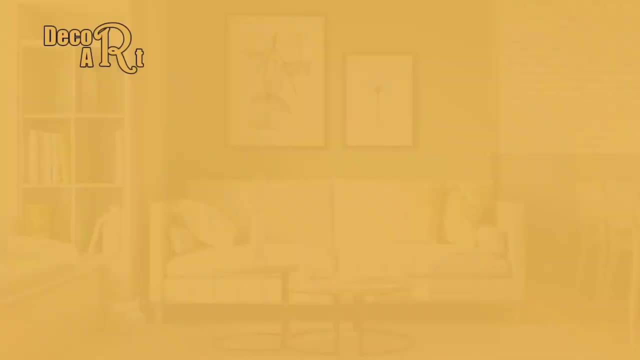 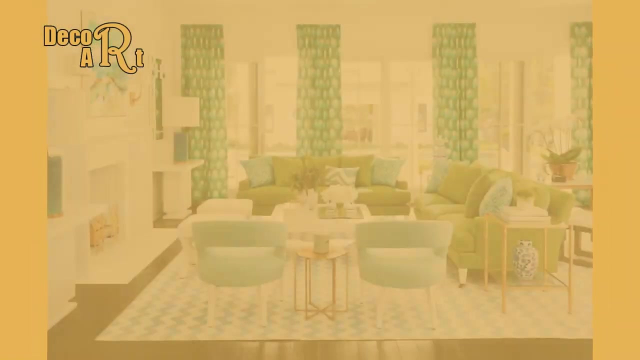 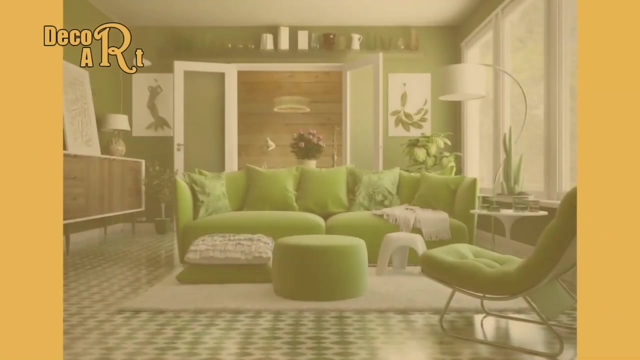 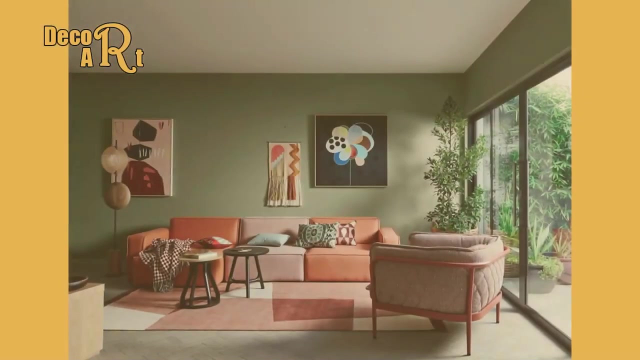 plants and green flowers. decoration is a fantastic idea, but do not overdo it. the most important characteristic of green color is its multi-purpose use. if you are wondering whether it will fit your space, the answer is usually yes, whether it's a green accent wall or a few see form green throw pillows, adding a pop of. 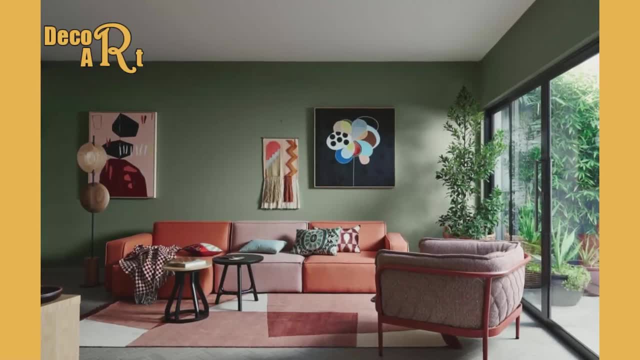 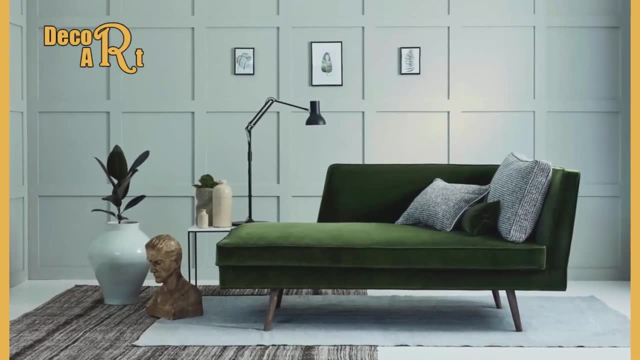 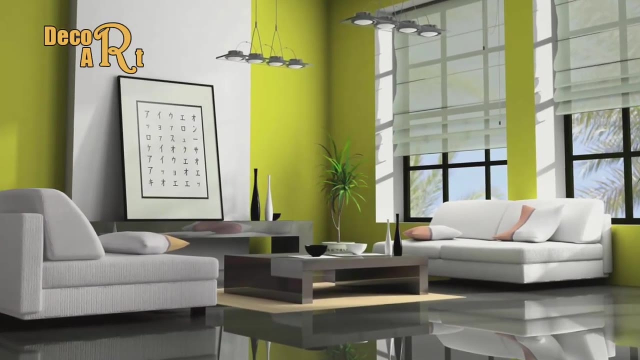 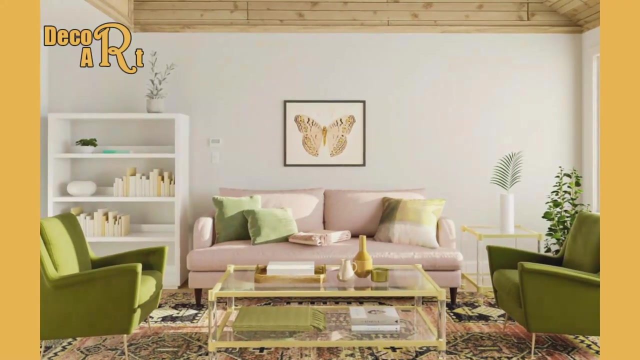 green has a power to completely transform any room. if you want a more dramatic feel, be sure to indulge in colors like dark moss and emerald green. looking for a little tranquility, paint your walls in a soft tissue like mint. and for those looking to make a big impact, there is always the tried-and-true lime green. if 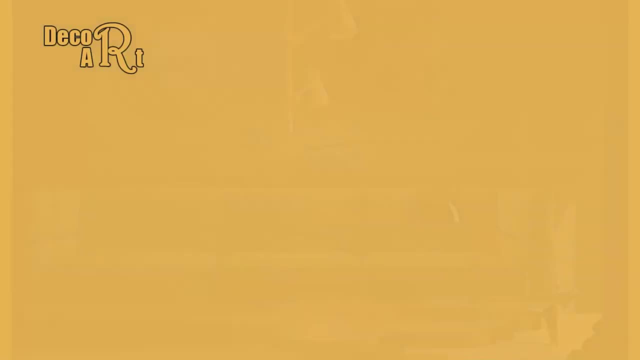 you're not quite sure which color best suits you? we've got you covered. keep scrolling to see our hand-picked collection of the best green living rooms by designers and visualizers around the globe. at the end of this video, please like comment with your favorite design share. 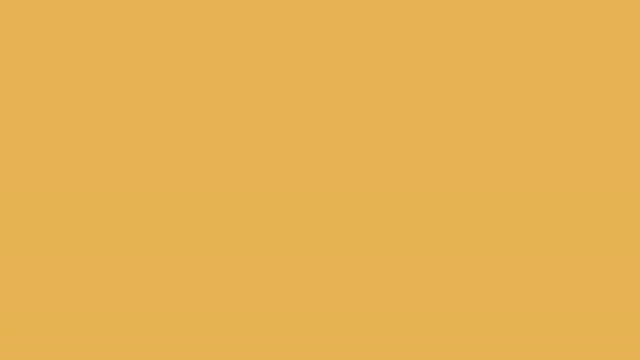 it with your friends and subscribe to our Channel.